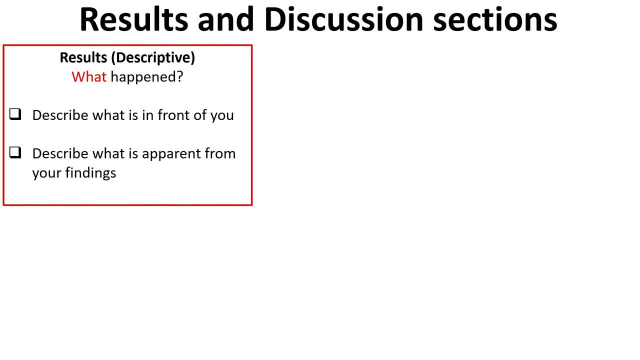 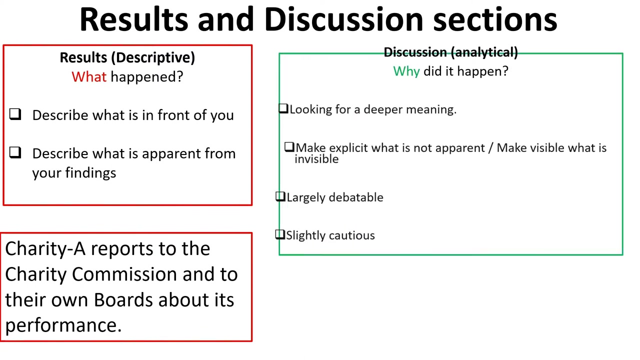 You are just presenting them or stating common facts about the organisations you are investigating, or providing background or contextual information. All of this is being descriptive. Here is an example of being descriptive. Charity A reports to the Charity Commission and to their own boards about its performance. very much on the surface. 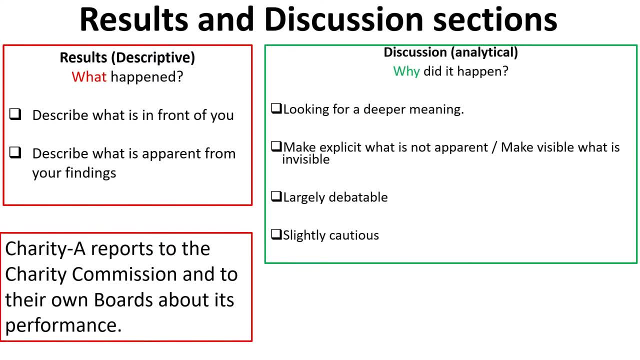 The opposite of being descriptive is being analytical. To be analytical is to find out why This is. when you look for a deeper meaning, You want to go below the surface. You make explicit what is not apparent. You make visible that which is invisible. 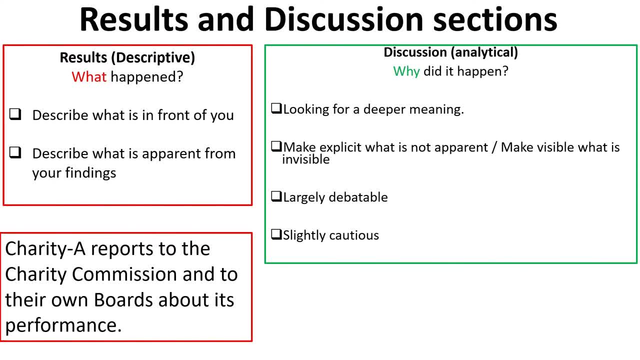 You want to suggest reasons that are not explicit. You want to be evident, You want to read between the lines of your interviewees comments, You want to explore the unsaid or you want to elaborate on their comments. Being analytical is to present points that are debatable. You may be right. 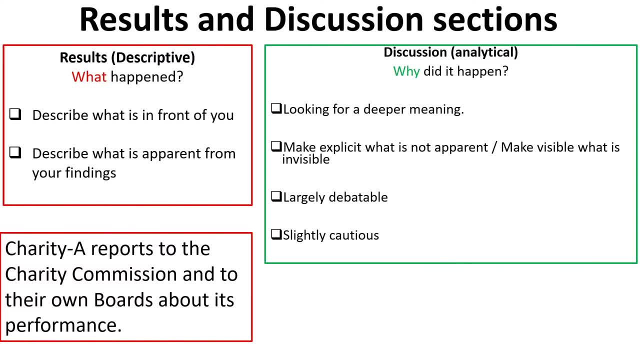 You may be wrong. Even though you are putting forward the most plausible reason, you can still be wrong. Being analytical is not an exact science. Since you may be right or wrong, your writing is always cautious. Tread carefully. Arguably, it could be that Possibly it may be because 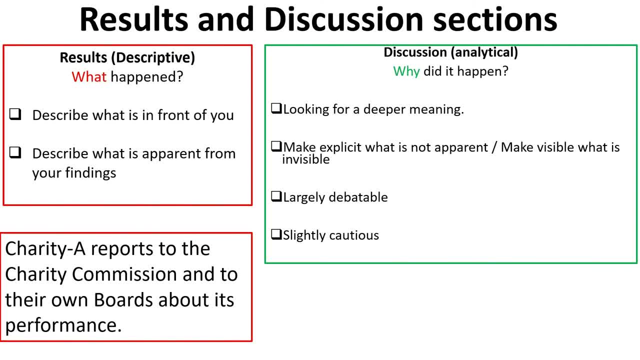 It could be due to this. It could be due to that The language is always very cautious, because you may be right or wrong. An example of writing analytically is the way in which Charity A reports its performance can be seen through the lens of legitimisation theory. 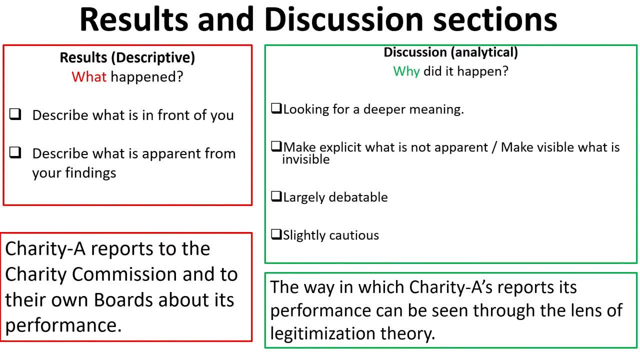 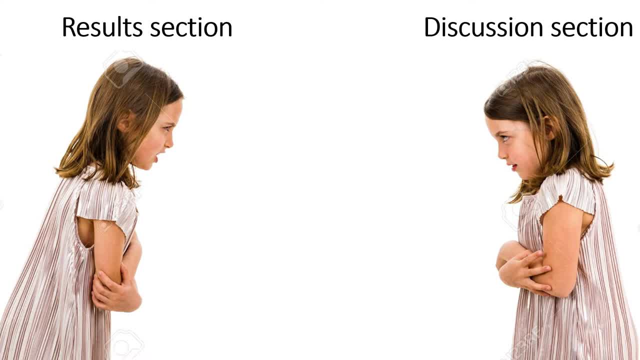 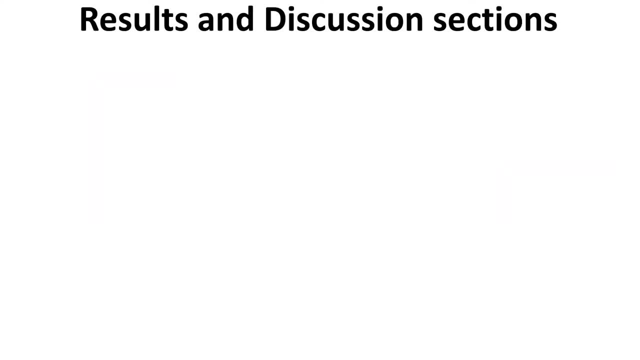 You are seeking to offer a deeper view of an apparent action. There is also another difference between the two sisters. The results section requires you to specify, while the discussion section requires you to generalise. In the results section, you should describe the content of your interviews, surveys or questionnaires. 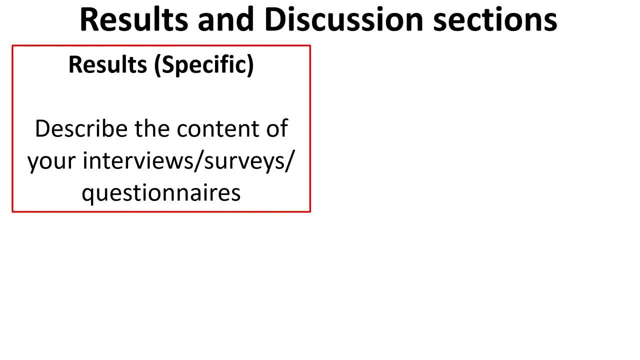 Your focus is on the specific words and deeds and actions of interviewees, respondents or organisations. An example of this is the following: An example of this is that the interviewee felt that the care staff had a negative attitude towards her because of her age. 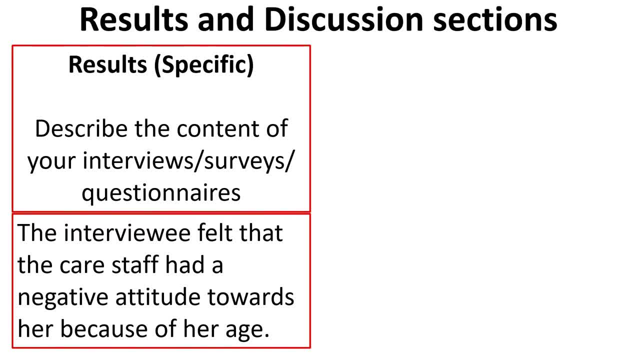 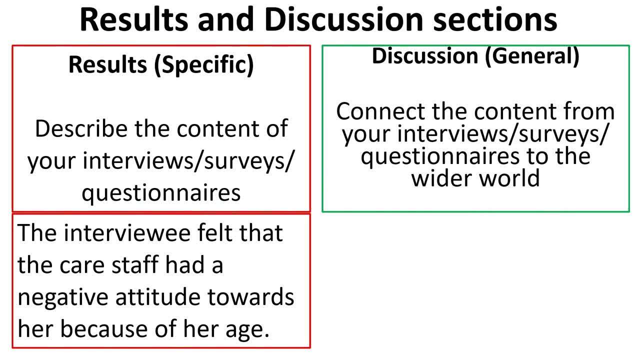 Presentation of this specific observation is central to the results section. In contrast, the main job of the discussion section is to connect the content from your interviews, surveys or questionnaires to the wider world. How does the words, deeds and actions you presented in your results section? 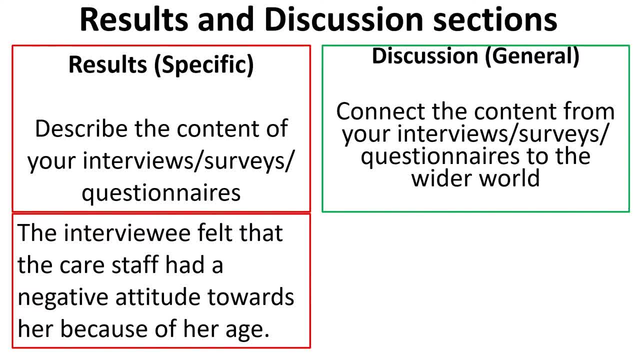 relate or impact wider society. You'll find that when you want to publish your research, editors want you to discuss the specific nature of your data, But what they really value is that you connect your specific data with the wider society. Scholarly activity of connecting, correlating, associating, establishing relationships is highly valued. 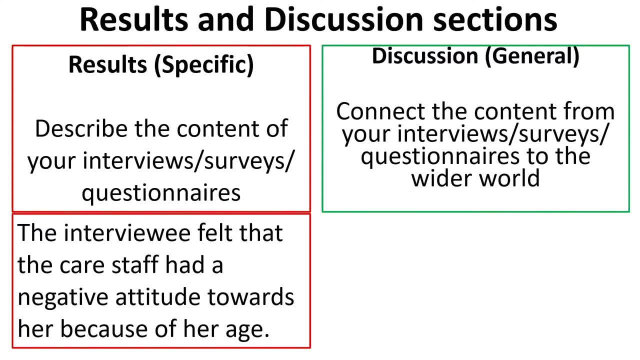 However, make sure, when you generalise, that you cite or reference the literature. This will make your generalisation stronger. Also, when you make connections, use cautious language and be conservative. Do not make exaggerated claims. An example of a discussion is that in the results section. 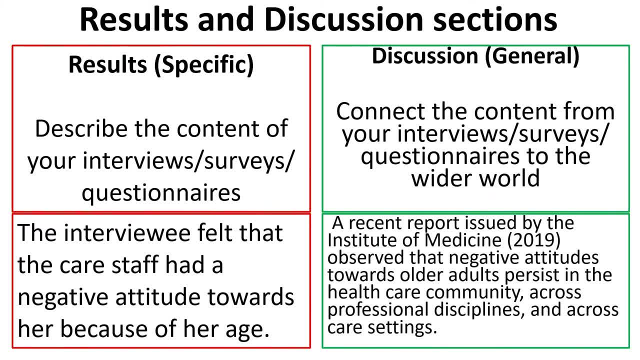 you talked about your interviewee experiencing negative attitudes because of her age. You now connect the data. You now connect that specific experience to wider occurrences. This was not an isolated incident. Rather, a recent report issued by the Institute of Medicine observed that negative attitudes towards older adults persist in the healthcare community. 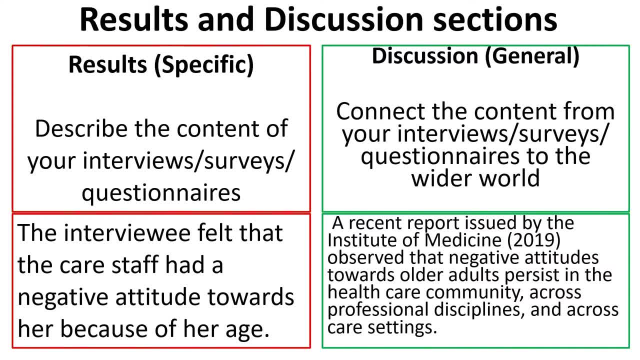 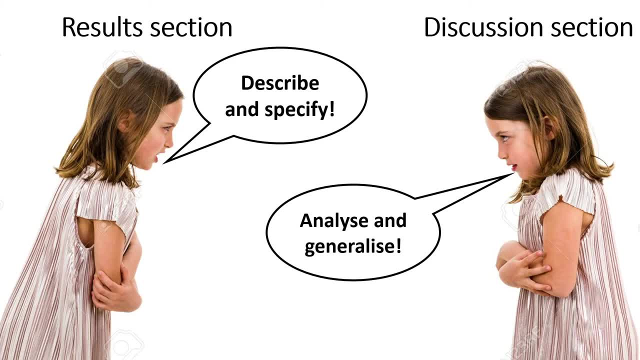 across professional disciplines and across care settings. It could be a specific observation or off-handed comment or phrase, or even something unsaid from your interviewees. Then you try to connect that with the wider trends or wider occurrences. It is important to note that I have described the general character of the results section. 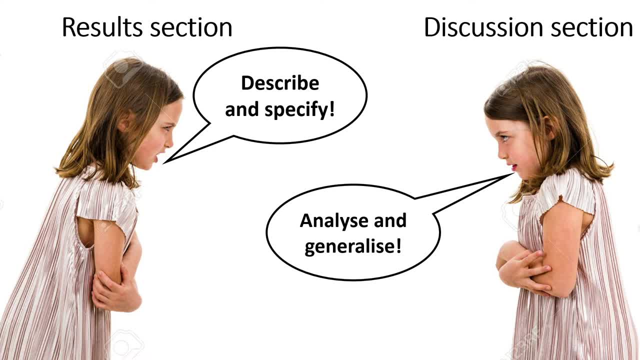 and the general character of the discussion section. You may find that in the discussion section you may need to describe certain things, Or in a results section you may need to analyse certain things, But make sure the general character and the general nature of the discussion section. 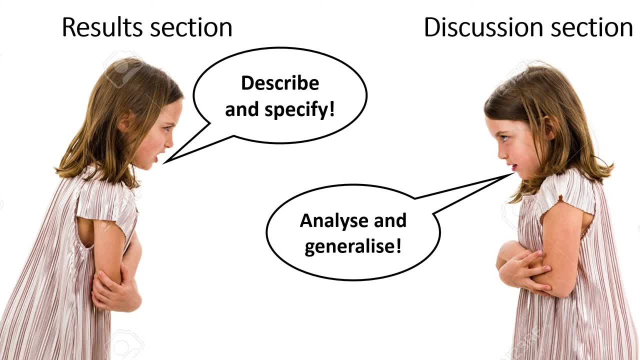 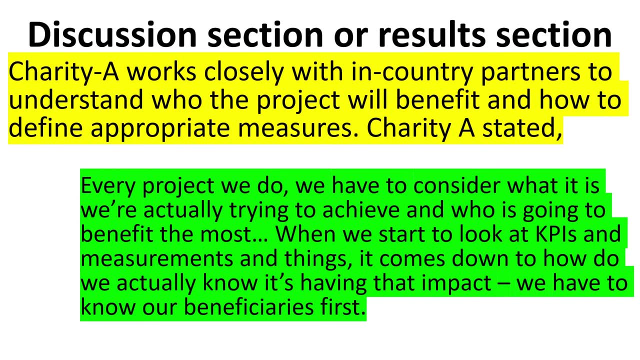 is analysis and generalisation And the general nature of your results section is specification and description. So I have here an activity. Would this sentence be typically found in the results section or the discussion section? Notice the intro sentence in yellow and the interviewee statement in green. 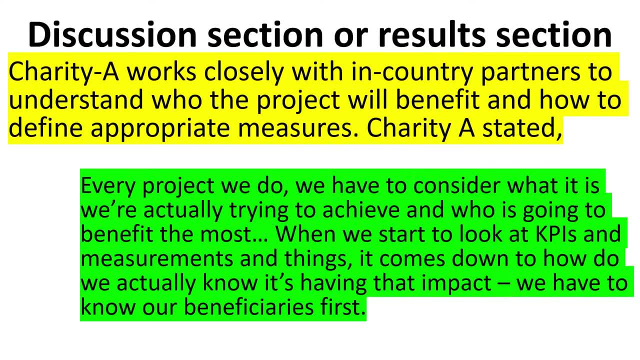 The author of this dissertation has described what the interviewee statement is about before they show the interviewee statement. Whenever you present a statement or quantitative information, explain what it is. first, Make it easy for the person marking your work to know what is happening. 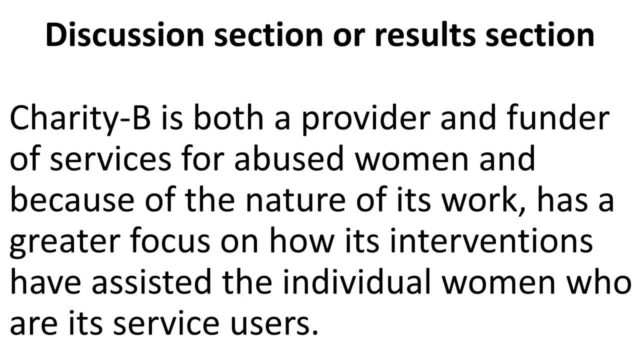 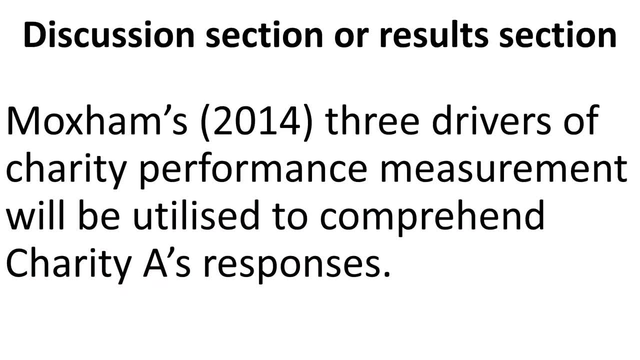 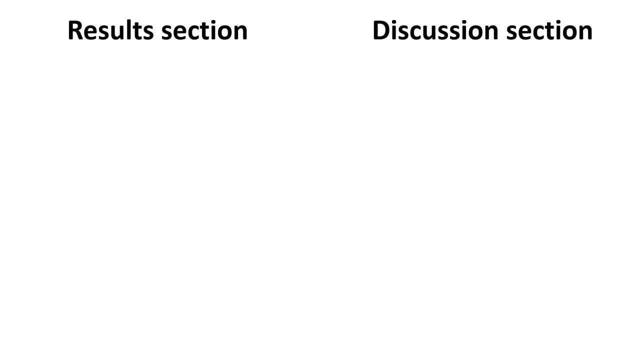 Would this sentence be typically found in the results section or the discussion section? Would this sentence be typically found in the discussion section or the results section? I want to show you now how the results section and discussion section mirror each other. In the results section, you may have a subheading like this: 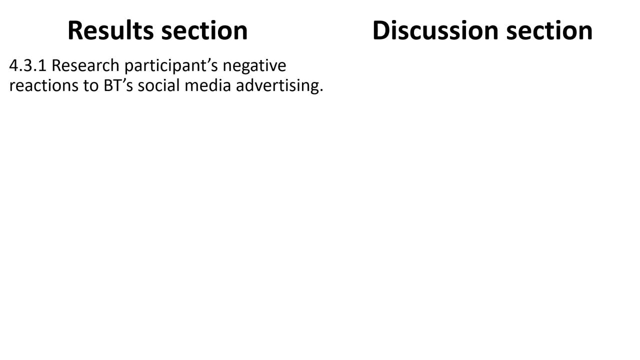 Research Participants' Reactions to BT Social Media Advertising. This is a descriptive section where you just present the research participants' reactions to BT social media advertising. Research Participants' Reactions to BT Social Media Advertising. However, in the discussion section you return to this theme. 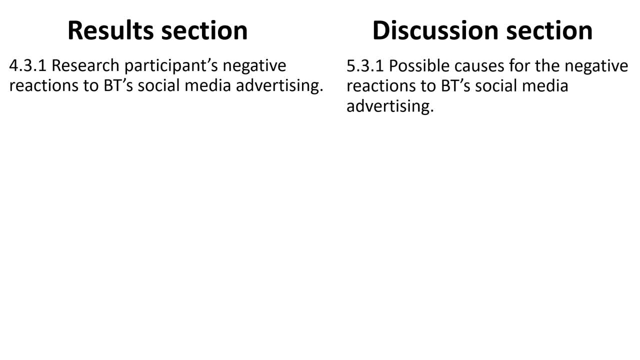 but you analyse it this time around. You try to figure out the possible causes for the reactions to BT social media advertising. Which theories explain the reactions? Which contextual or structural reasons explain the reactions? You have discussed the what in the results section. Now you want to discuss the why in the discussion section. 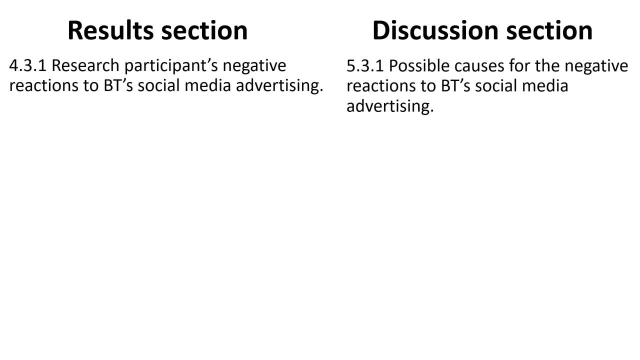 So in both the results section and the discussion section you are looking at the same theme but you approach it in two different ways: The what and the why. Also in this discussion section you are generalising. In the results section you discuss specific reactions. 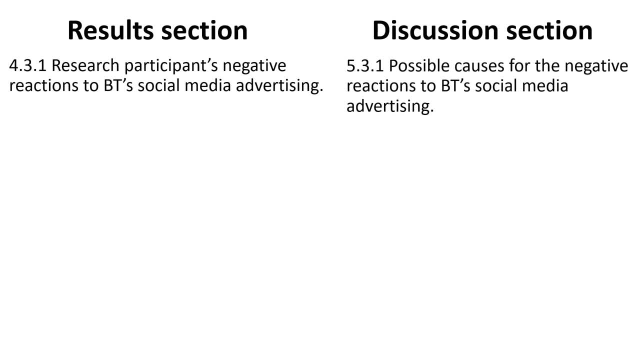 to BT social media advertising from the individuals you personally interviewed. Now in this discussion section you want to try to make general connections between those people that you interviewed with the wider reaction in wider society. The possible causes that you are writing about are the possible causes for the wider society. 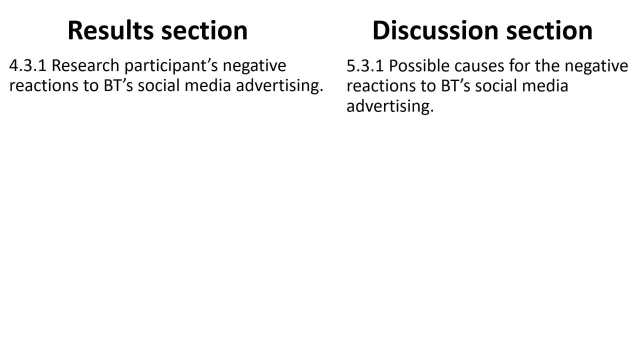 not just that small group of people that you personally interviewed. One more example: In the results section, you presented students' comments on their experiences with the supervision process. You selected the most important comments from these students. You will now analyse these comments or unpack these comments. 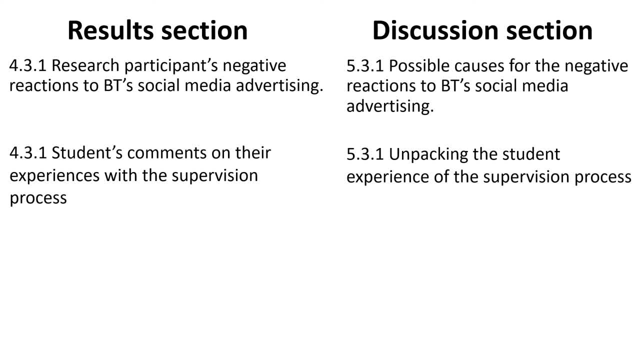 What is behind these comments? Which factors encourage these comments? Do these comments agree with something you've read Or do they contradict something you've read? If so, what are the reasons they contradict the literature? These are typical analytical questions In the results section. 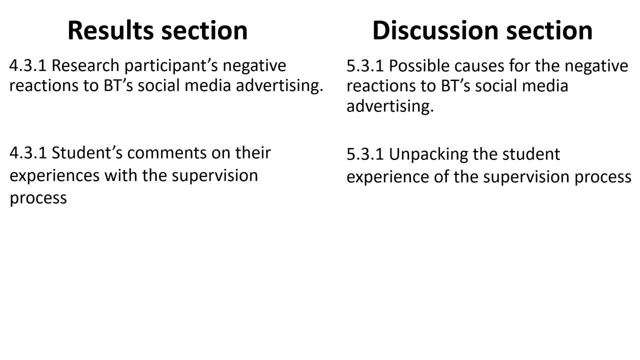 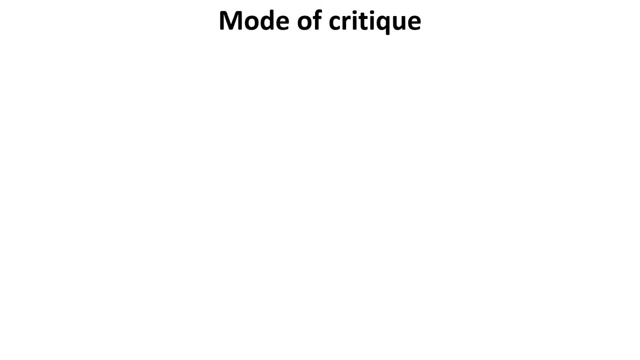 you discuss the specific individual student experiences from the students that you interviewed, But in the discussion section you discuss the broader student experience. The concept is abstracted. now, Throughout this video I've explained the macro approach, That is, you separate the results section. 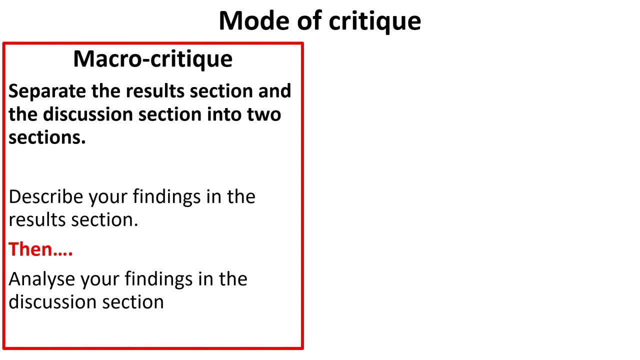 from the discussion section. They are essentially two distinct sections. The results section is about three to four pages, followed by the discussion section, which is about five to six pages. This is the most common approach. I prefer this approach because it is less messy. 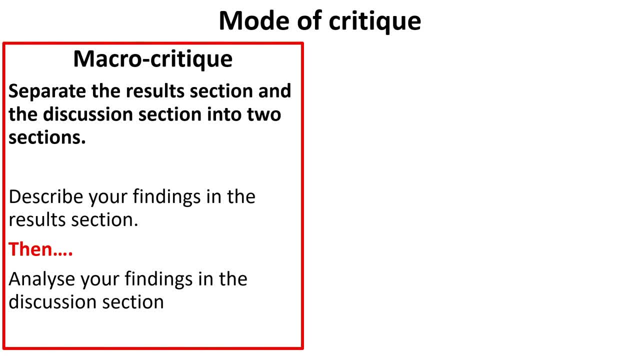 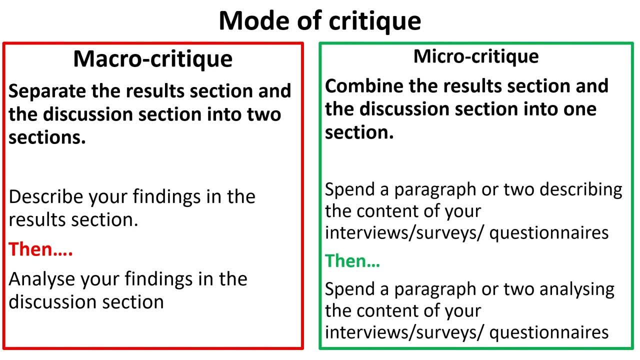 It is very clean: The results are over here and the findings are over there. However, there is another approach, The micro approach. This is where you combine the results section and the discussion section into one section, So under a subheading. 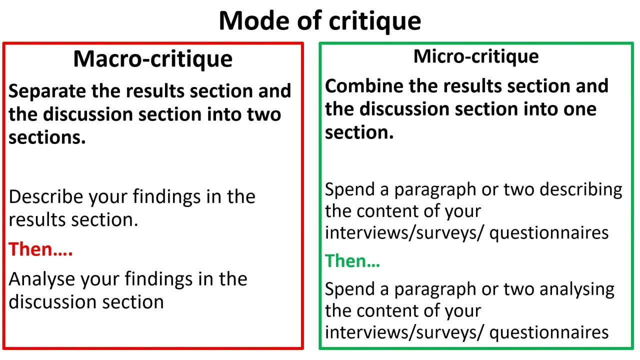 you describe a particular theme from your interviews or surveys or questionnaires, This is immediately followed with an analysis of that same theme. Simply put, one or two paragraphs describing, followed by one or two paragraphs analyzing Present content from your interview, surveys or questionnaires.